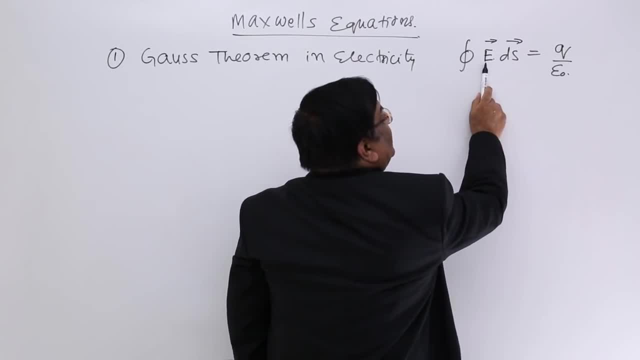 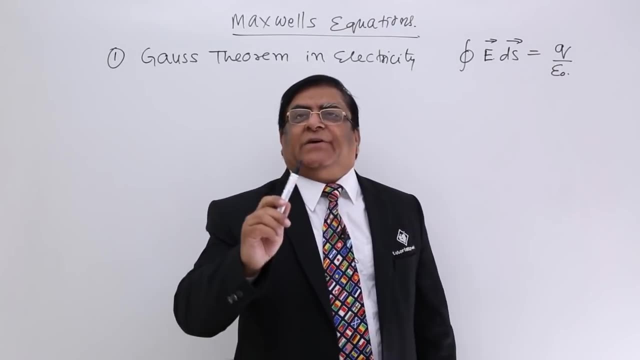 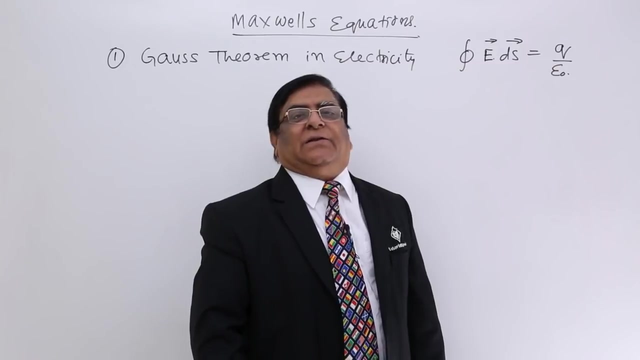 publisher of well, intelligent chip In both this section, this equation field. and wherever there is electric field, it cannot exist, electric field, without its source q. So whenever there is electric field, here I need not ask: is there any charge? because I know electric field cannot exist without a charge. it cannot be created, there has to. 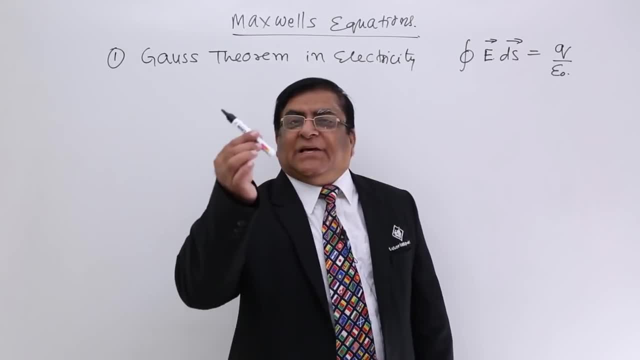 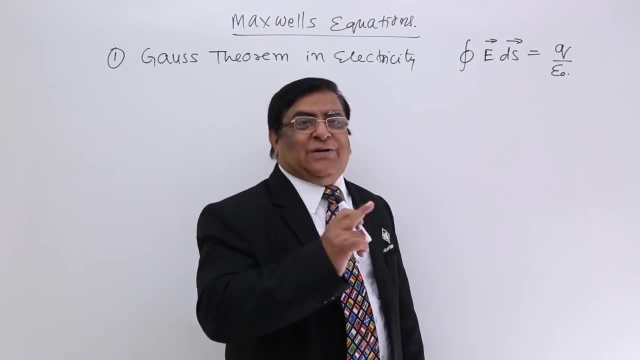 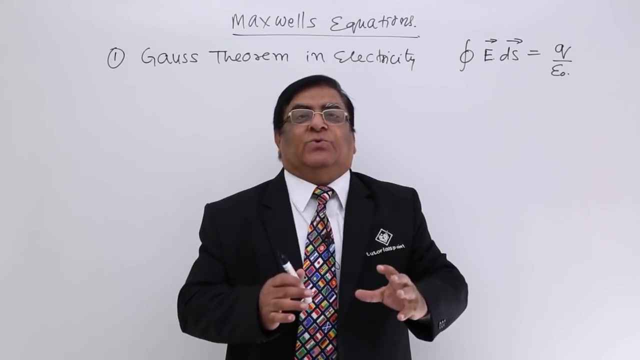 be a charge. Similarly, if there is a charge, we cannot ask: is it creating an electric field? no, we do not need to ask it because any charge will always create an electric field and the relationship between the two. how much electric field is created if we cover a charge around? 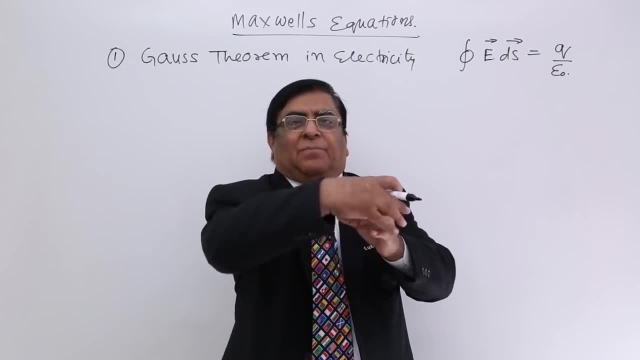 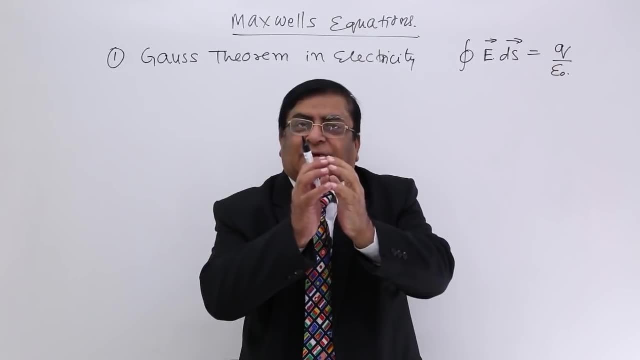 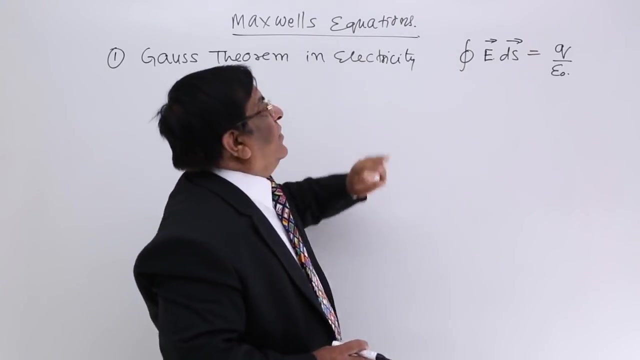 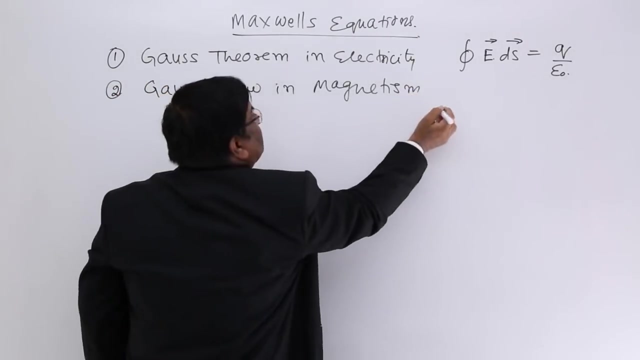 it with a surface area, then electric field multiplied by surface area that gives us the quantity of charge. more is the charge, more is the electric field. increase the surface area, then intensity will decrease. all these things we have studied In Gauss theorem of electricity. second, we have Gauss's law in magnetism. this is closed. 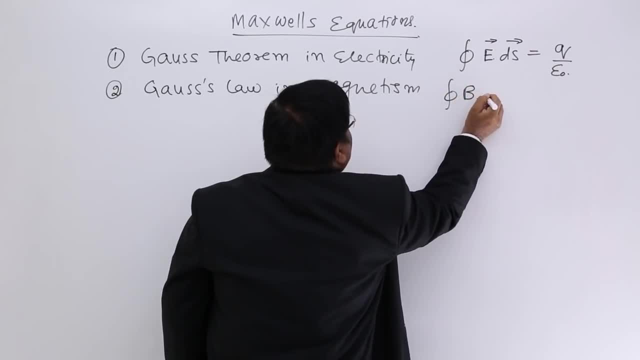 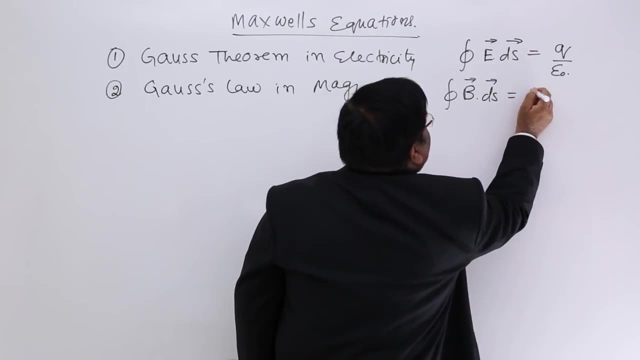 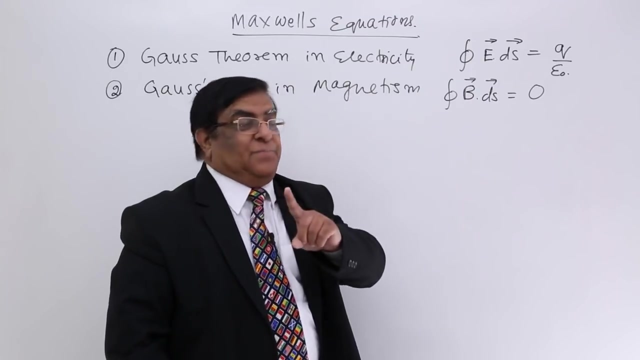 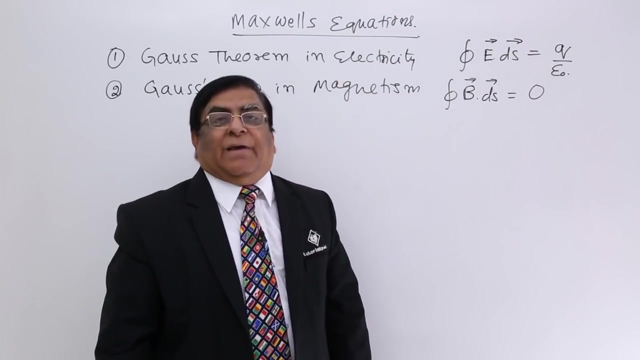 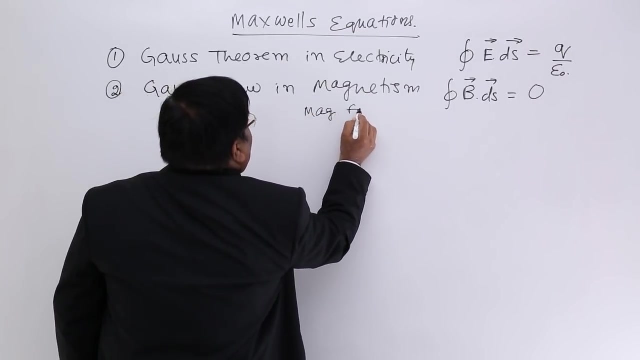 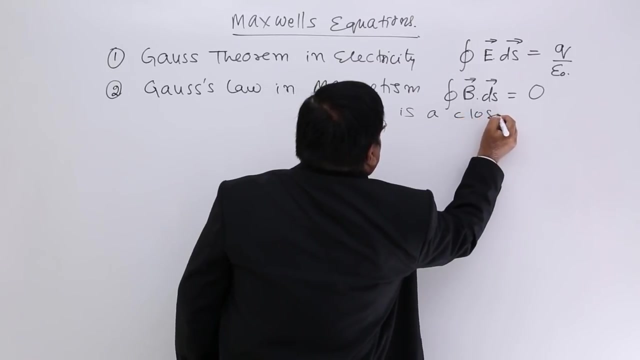 integral B ds in place of E, it is B closed. integral B ds is equal to 0. nothing, how it is so important. It is important. It says That magnetic field is always a closed line. Magnetic field is always a closed line. Magnetic field is: or magnetic lines is a closed field, or the magnetic lines are closed field. 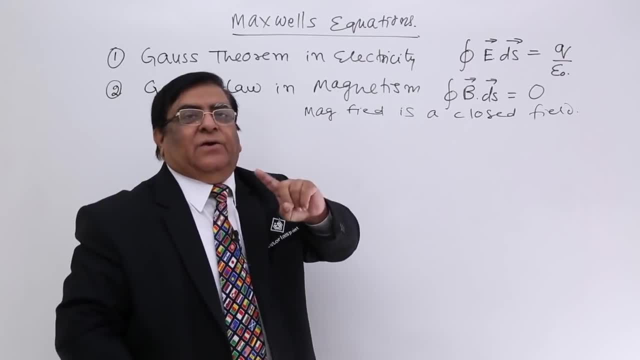 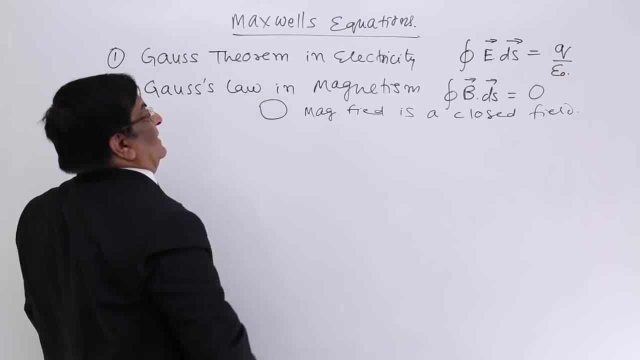 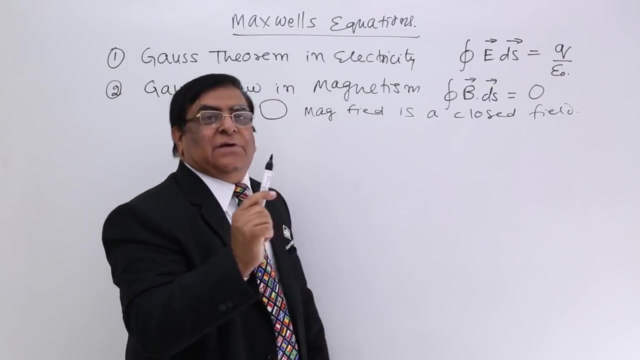 lines. There are no, We have seen it. There are no starting point, There are no termination for the magnetic field and they are always ending at the same point. so they are incomplete circle, in contrast to electric field, which starts from positive charge and terminate at the negative charge, wherever there is a positive and negative. 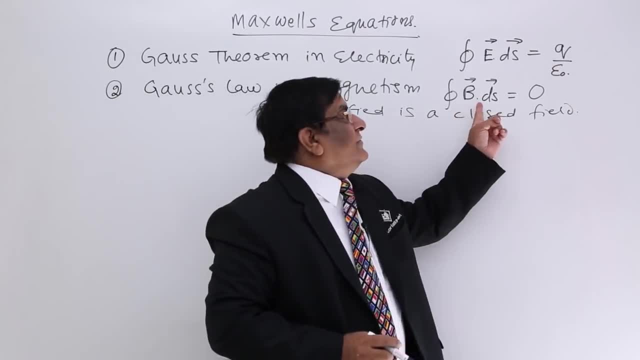 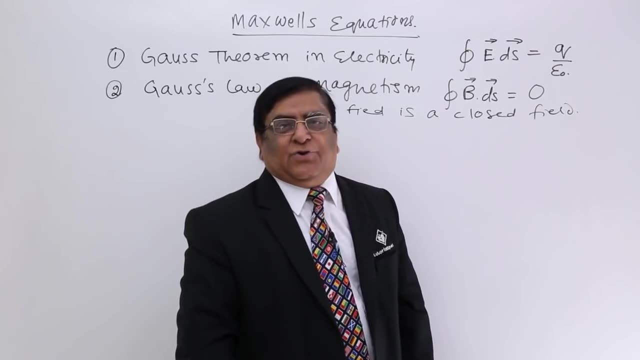 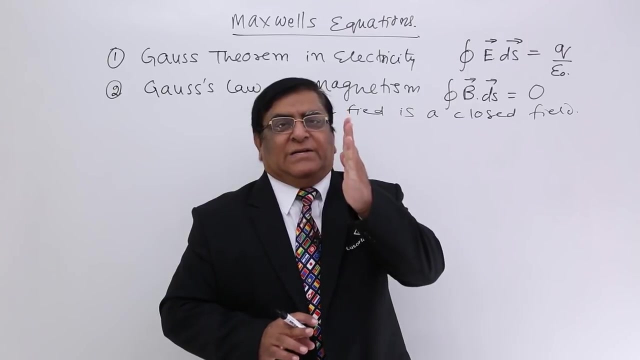 charge. then it also states that our earlier thinking that there is a north pole and there is a south pole, that was not correct. there is nothing, no entity, known as North Pole or South Pole. It is only one, same source, which is observed from both the sides. 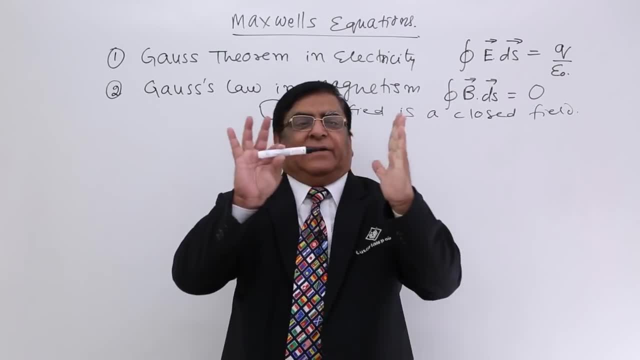 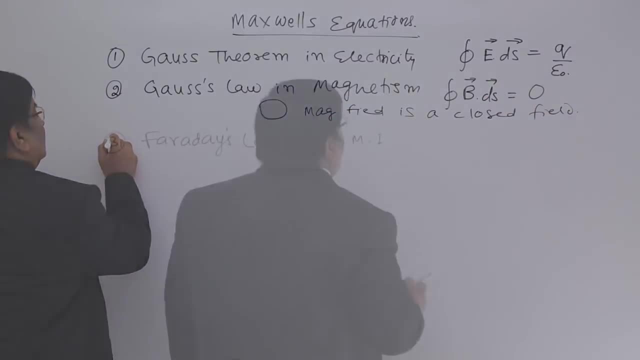 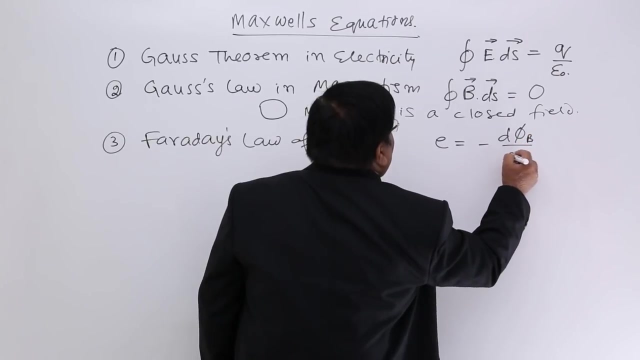 From one side it appears to be North Pole and here it appears to be South Pole. All these things comes with this equation. Then, third equation, Faraday's law of electromagnetic induction. we have studied that E is equal to minus d phi by dt. 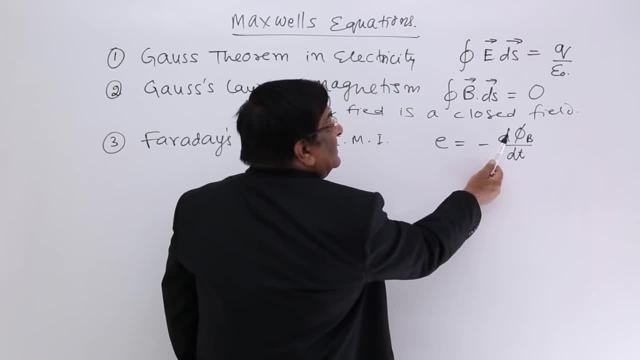 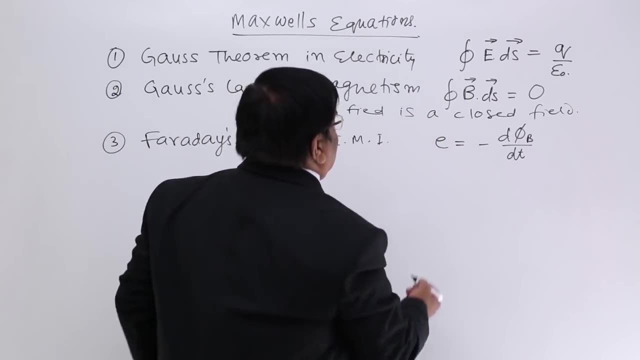 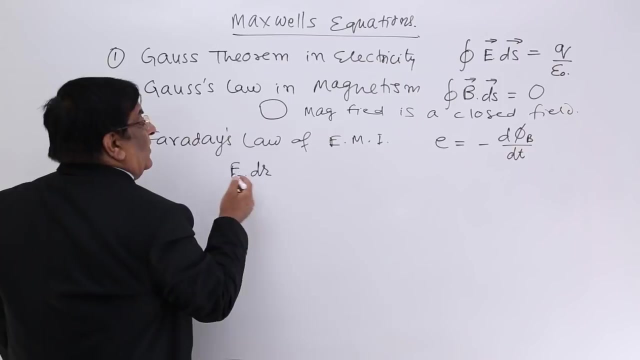 What is this? Rate of change of magnetic flux? rate of change of magnetic flux is equal to emf induced. Now, if we expand it a little, emf is what voltage? and voltage is equal to E, dr or Edl. whatever you say, this is voltage, okay. 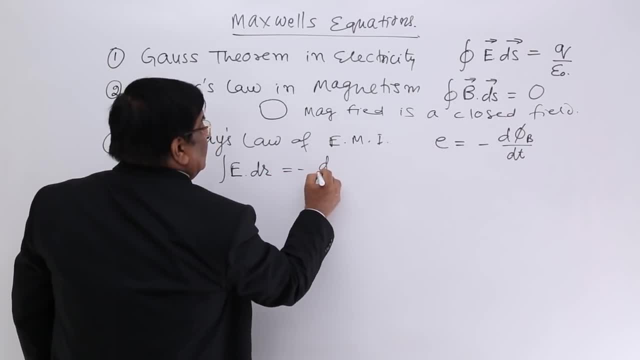 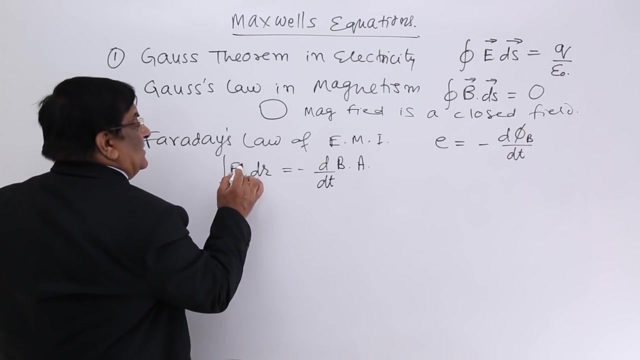 This is equal to d, phi by dt, d by dt of phi. What is phi Phi is b multiplied by a. okay, So here now you see, this is the equation format, and I draw your attention to these two quantities. One is E and one is this: db, dt. 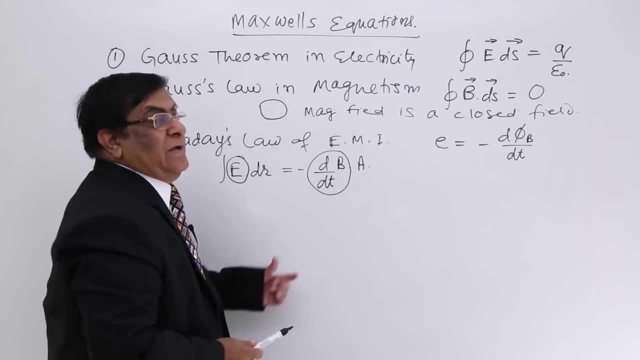 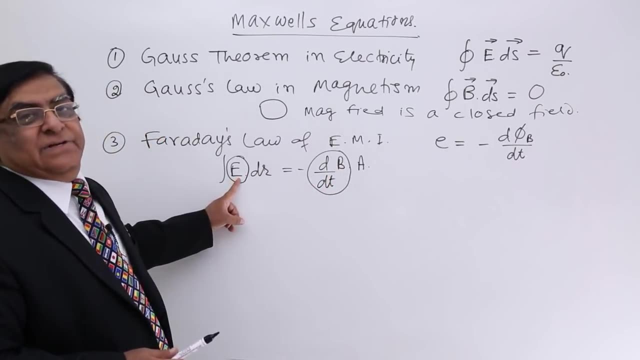 These are constants. we can leave them. This gives us a very important result. Whenever there is a change in magnetic field, we always get an electric field. This is electric field, this is magnetic field and it is changing d by dt. 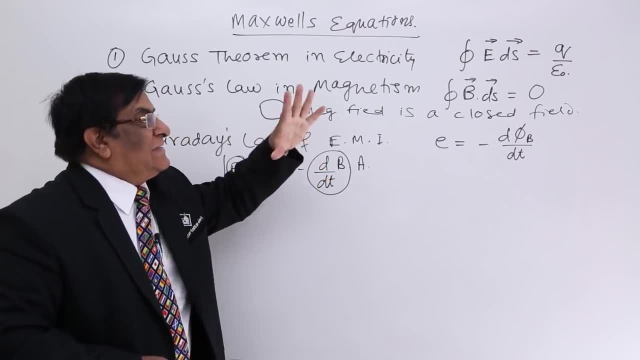 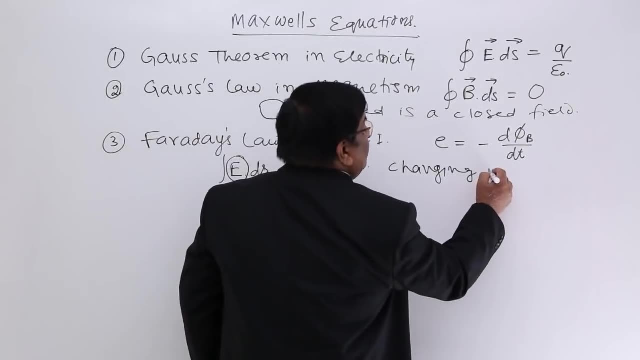 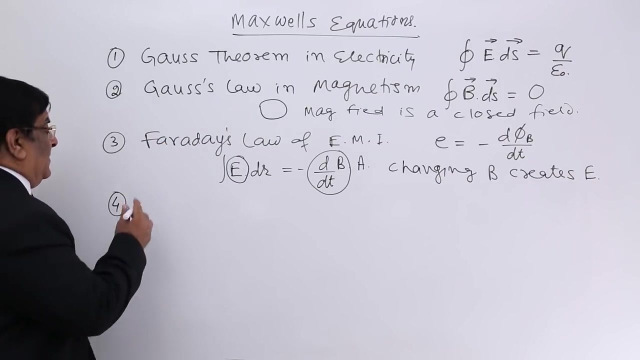 Whenever there is a change in magnetic field. if magnetic field makes like this, it will create an electric field. This is the relation. Faraday's Changing b creates the fourth equation, which was made by amperes and volts. This is the equation. 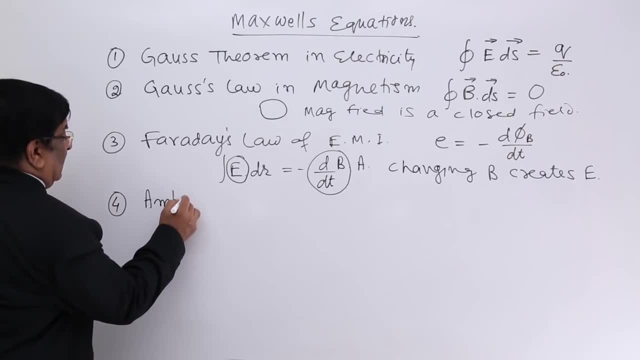 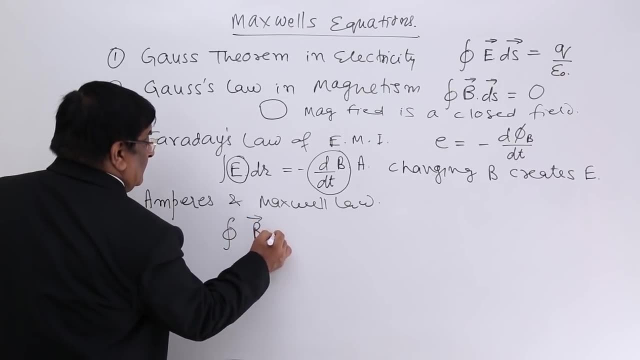 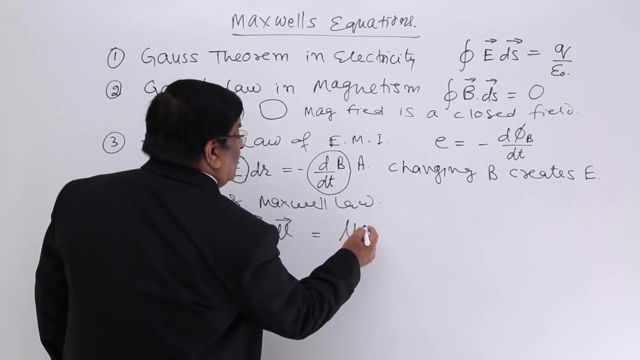 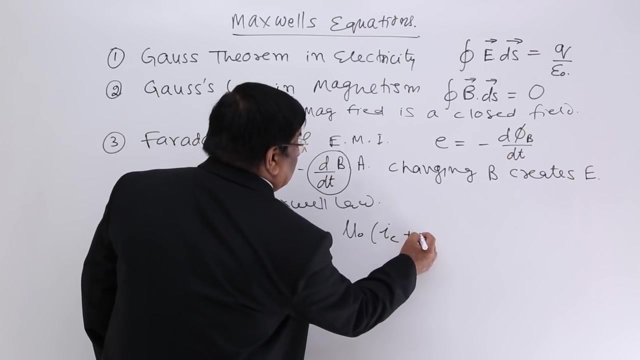 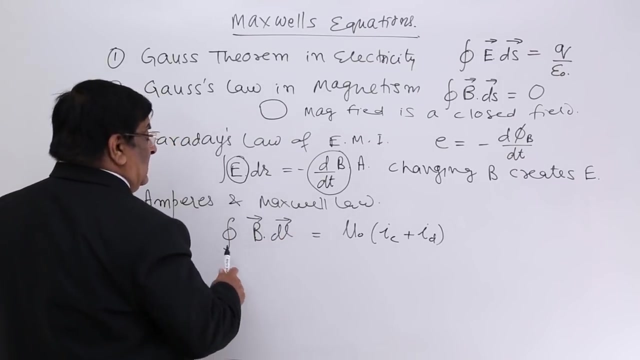 This is the equation Maxwell corrected by Maxwell: closed integral Bdl. Closed integral Bdl is equal to mu knot times current, and this current is I conductor plus I displacement. This is the equation, The corrected equation of amperes, which is known as amperes and Maxwell law. 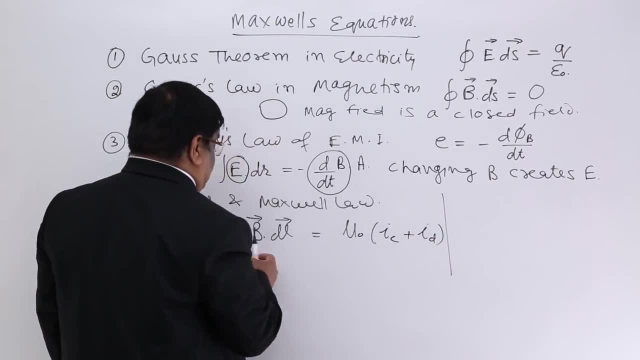 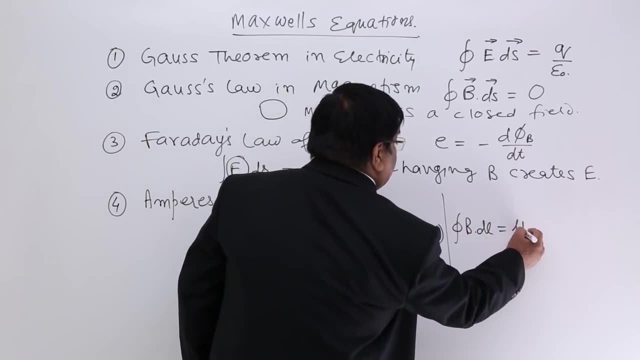 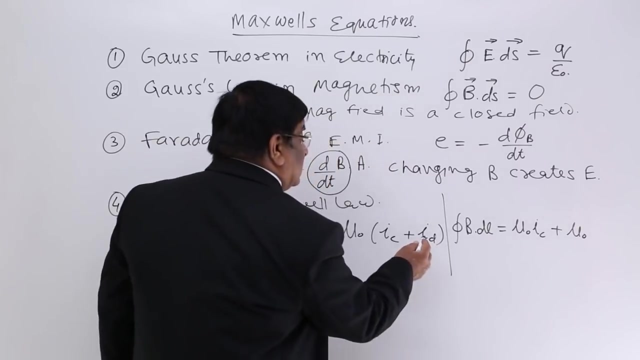 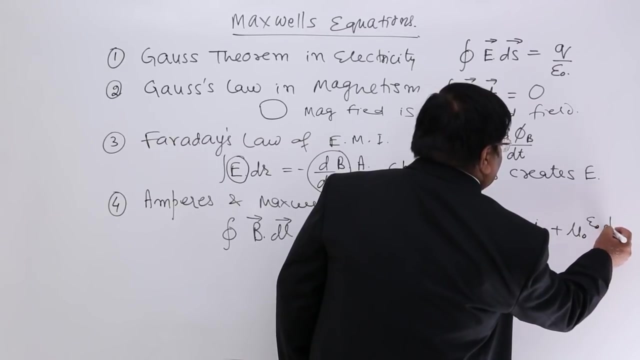 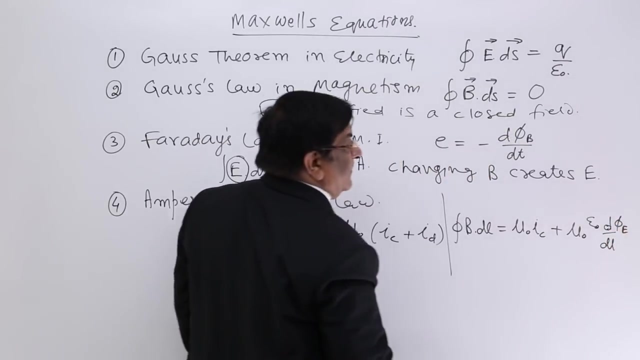 Now, if we extend this, what do we get? Closed integral Bdl is equal to mu knot Ic plus mu knot. This Id- we have seen It is epsilon knot. Okay, This is epsilon knot. But problem I have here is that to do a closed integral Bdl changeennis over E0 and change. 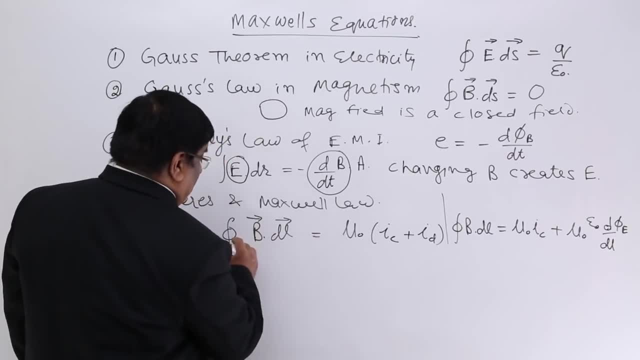 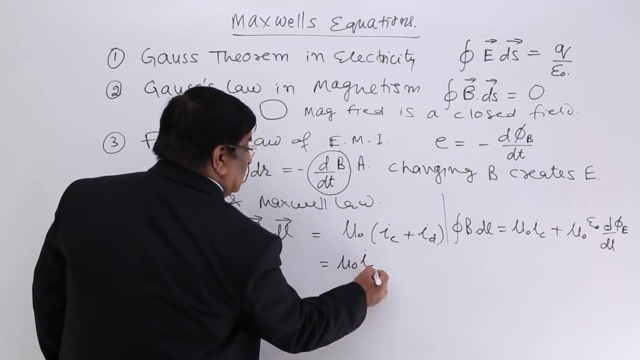 in electric flux. Electric flux. This again we can write as closed integral Bdl is equal to mu knot Ic plus mu knot Ic plus mu knot Ic plus mu knot II E0.. Which is it? It is closed integral Bdl. 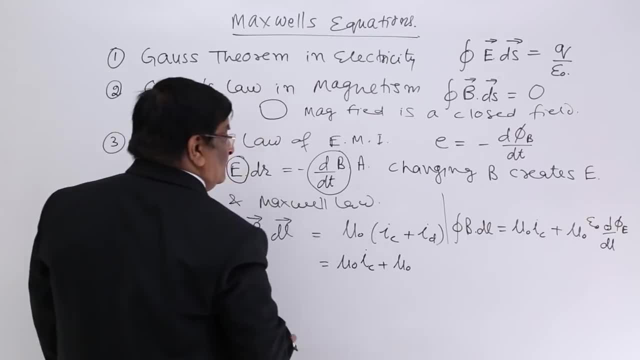 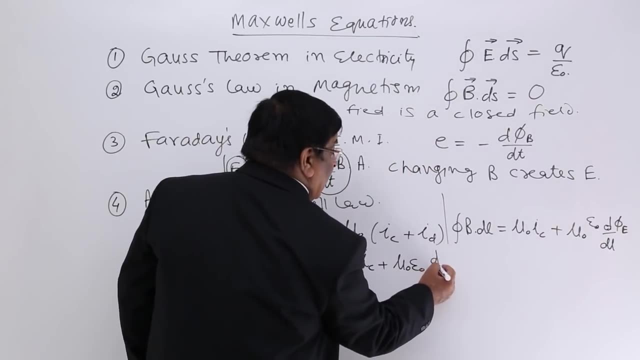 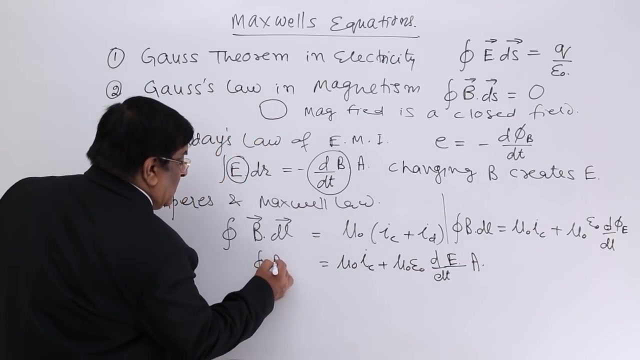 Close integral of Indigenous Executive is: must be equal to mu knot Ic plus mu knot 0, and here in d by dt of phi, e rate of change of electric flux. and electric flux is what Electric field multiplied by area. Now, in this equation, this is derivation from this. 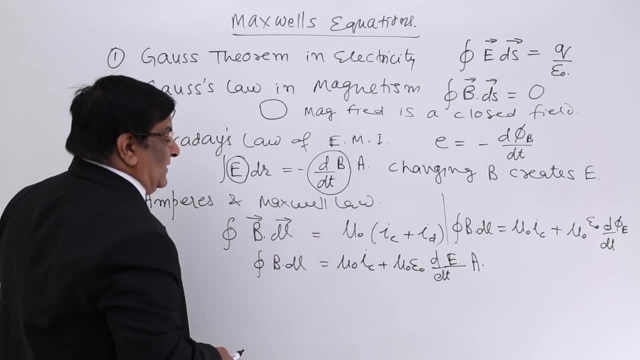 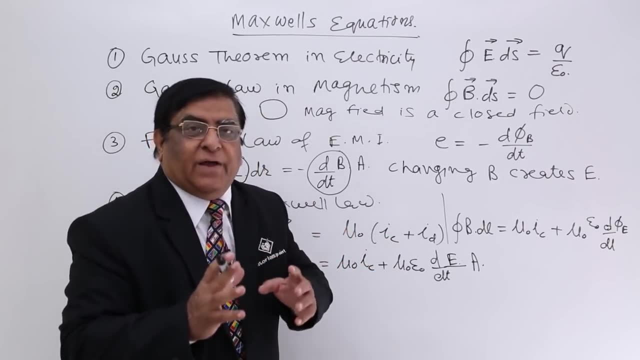 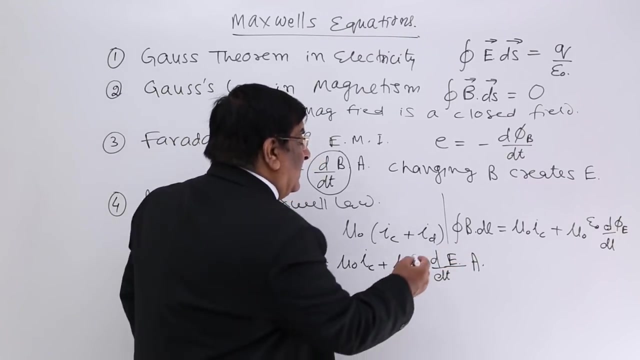 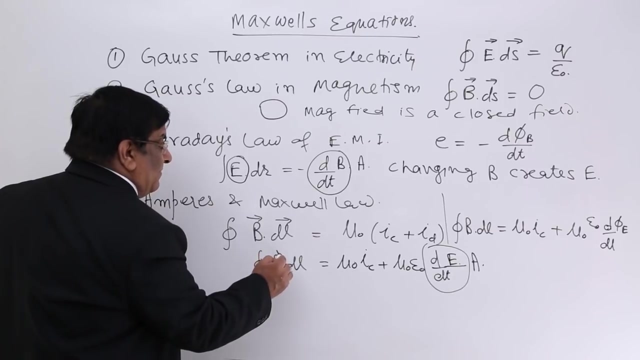 law. In this equation we observe one very important thing. This is, of course, current conduction, current at a space where an electric field is changing, and that mathematical expression is dE by dt change in electric field. What does it create? It creates a magnetic field. 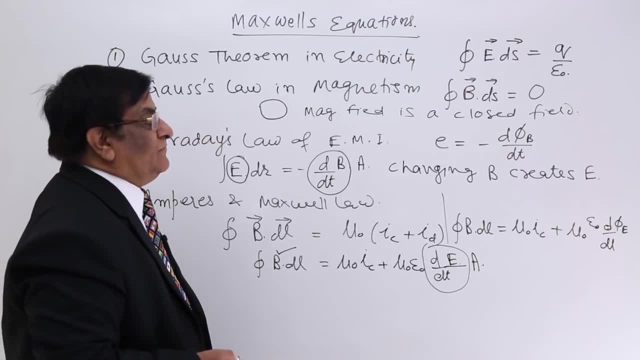 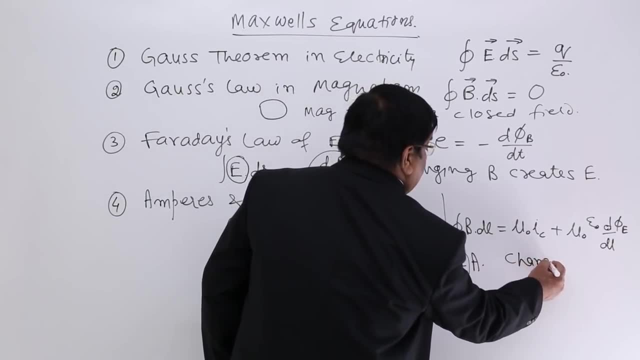 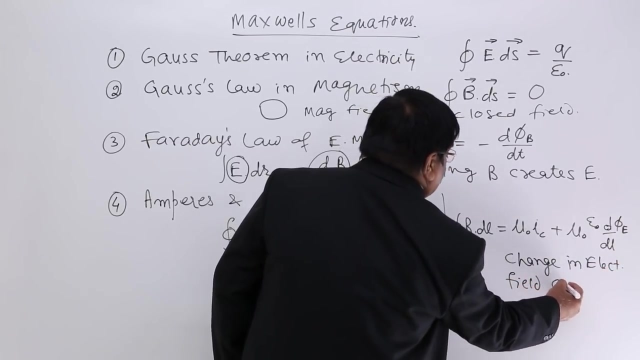 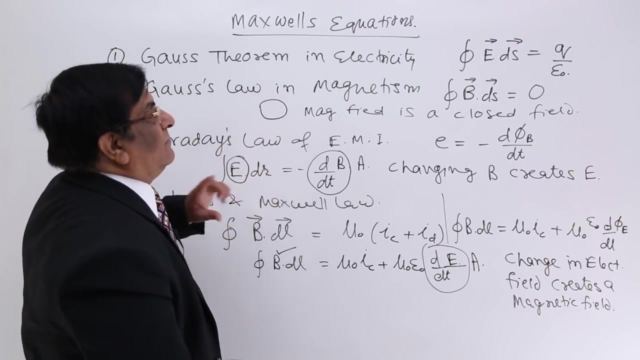 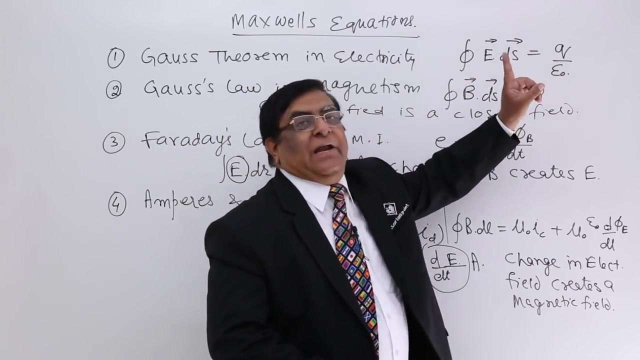 Change in electric field creates magnetic field. This is the important conclusion of Ampere Maxwell's law: Change in electric field create a magnetic field. So these are the four Maxwell's equations. I will repeat it once again: An electric field is created by electric charge. They: 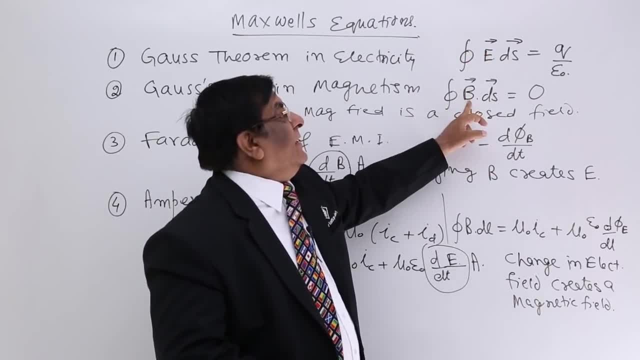 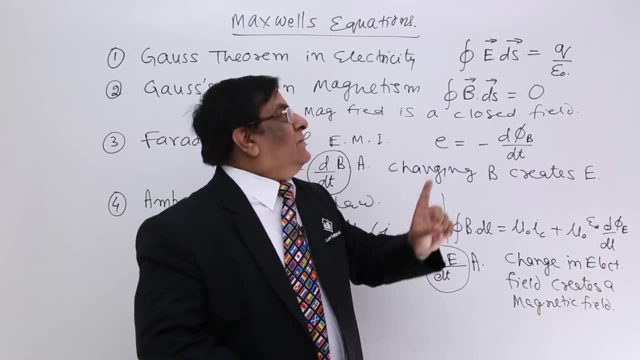 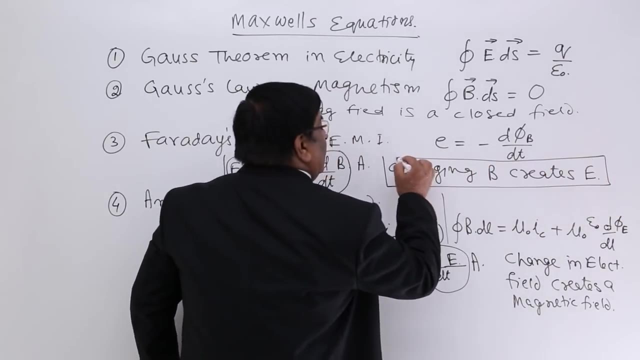 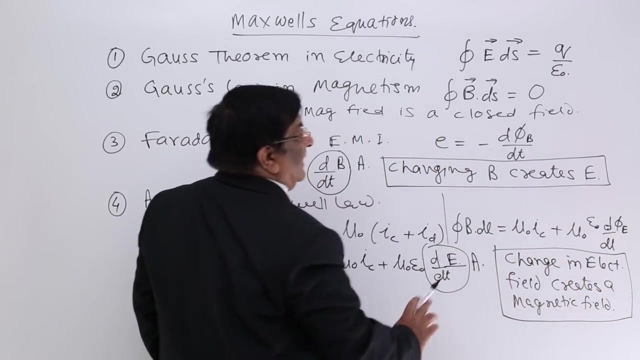 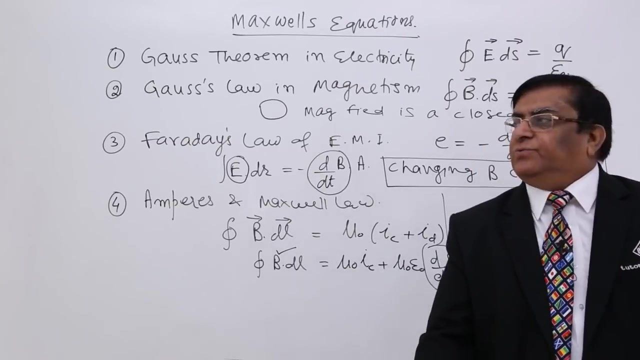 cannot exist without each other. A magnetic field is a closed field, always. There is nothing as north and south separate poles. Third thing: a changing, B changing magnetic field create electric field. and fourth is: changing electric field creates magnetic field. So these are the four general effects of the Maxwell's law which we have to remember for 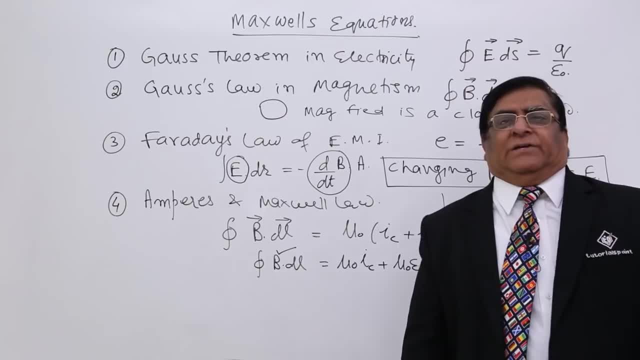 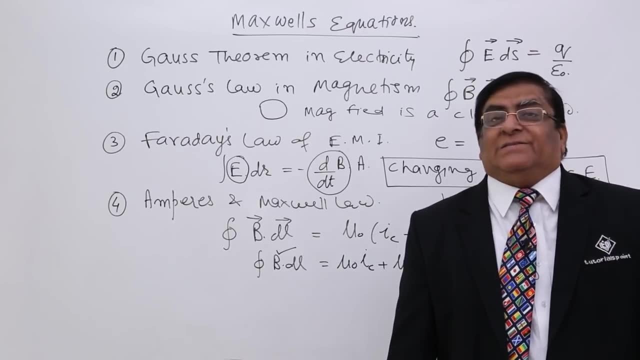 our standard. Maxwell did many, many calculations in a electromagnetic field and he is supposed to be the master of all. He is the one who proved that light is electromagnetic wave because of its velocity. He found, and again occurred, freenaire wives. They are입 seit PSykakis de, So there would 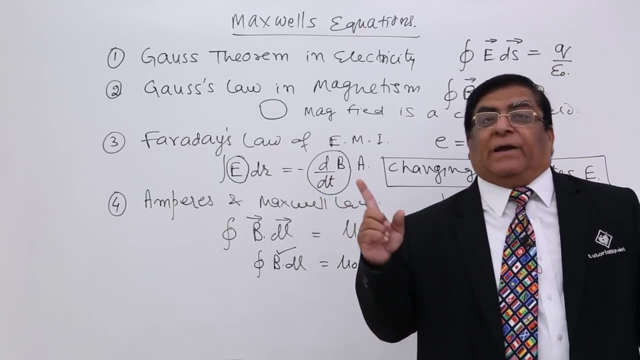 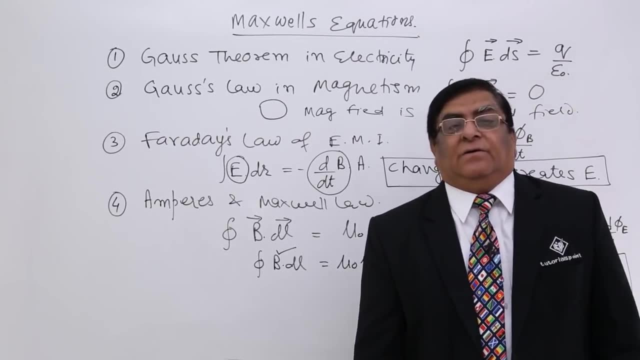 only be a little velocity between the right side and the left way, The right magnesii, the velocity of electromagnetic waves to be 3 into 10 to the power 8.. He is the one who said that electric field vectors in electromagnetic waves are transversal. Otherwise we used 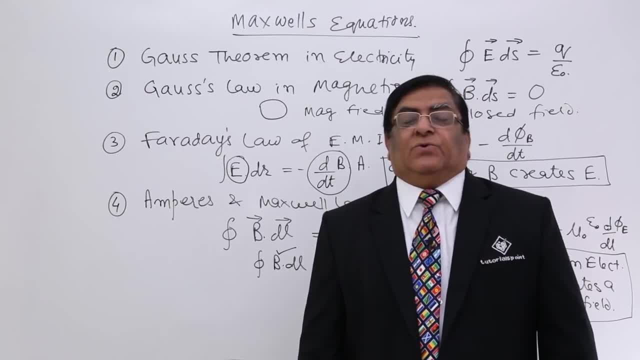 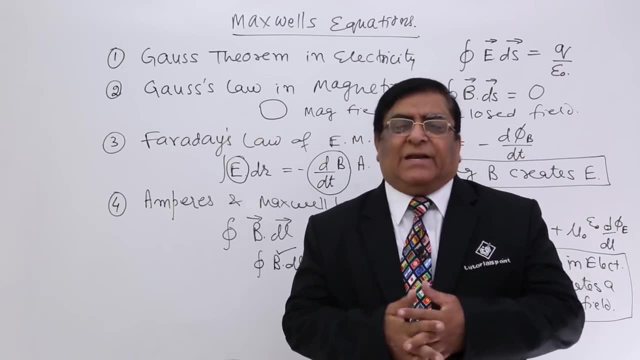 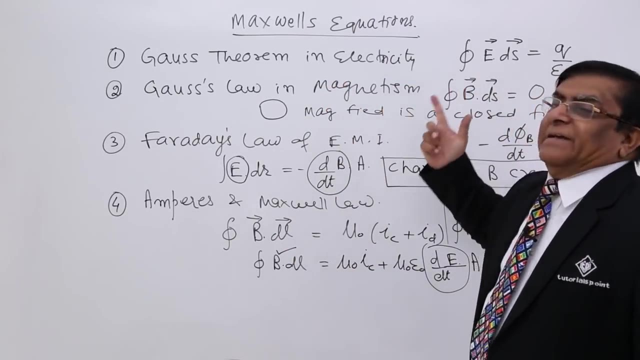 to think that they were longitudinal. So many credits go to Maxwell. So when we start studying Maxwell in this standard, we have to see only four equations. These were the four equations which are popularly known as Maxwell's equation. So then we will after. 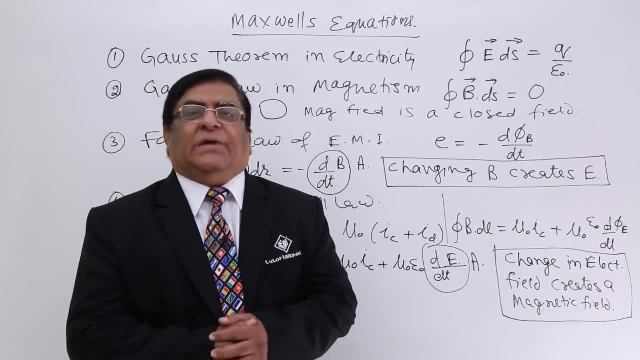 that we will study on the basis of this how we can understand the nature, the formation of electromagnetic waves. Thank you.